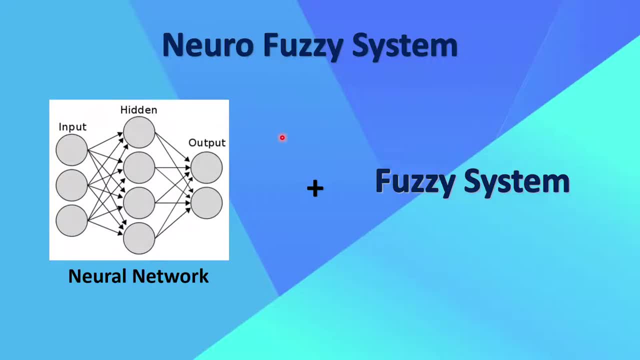 Hello future viewers, this is Praveen Soni. In this video I am going to talk about Neurofuzzy system. So let's start this. Neurofuzzy system is the combination of neural network and fuzzy system, where we are going to take some applications of neural network and the fuzzy system and 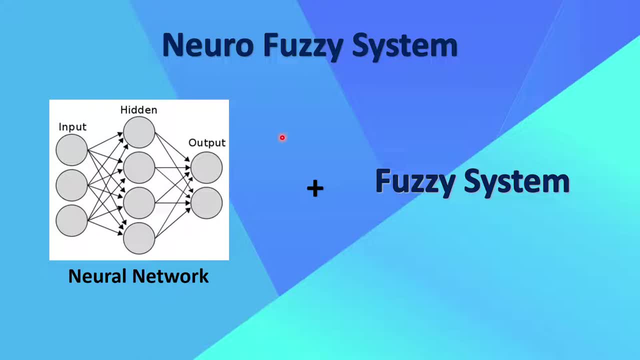 trying to combine both of them. As we already know, the neural network is the way to represent the neurons and in this neural network we try to mimic the human brain. And the fuzzy system shows the variation in the human brain thoughts and the thoughts that are present. 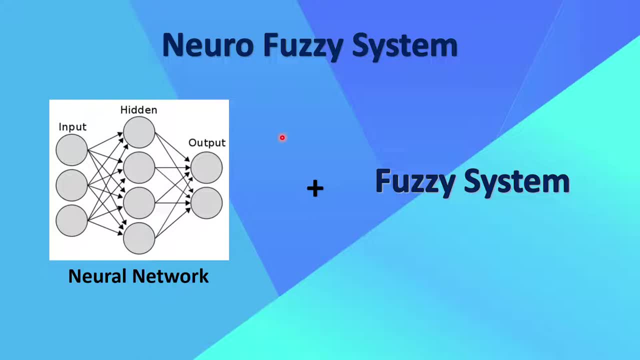 and all the variations that we have while we talk Or we give some statements. that is known as fuzziness. So in this Neurofuzzy system we are trying to combine both of them. So what actually the fuzzy is? So fuzzy means that 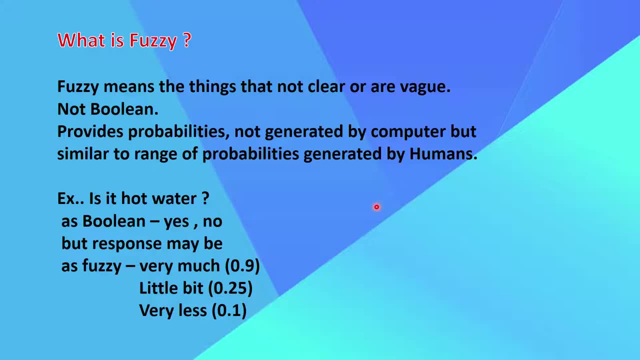 is the things that are not clear. For example, if I ask you: so what? how is the Taj Mahal? So your answer may be: Taj Mahal is a really beautiful place, Or it is a good place Or visit, But your answer will be not in the terms of true or false, like as Boolean. So 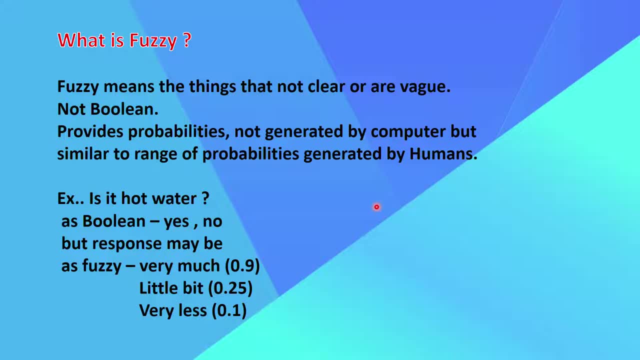 as our machines have a nature like Boolean: yes, true or false, true yes or no. So another example that I have mentioned here is that hot water. So in the terms of Boolean, the answer may be yes or no, But in the response, in the terms of fuzziness, the answer may. 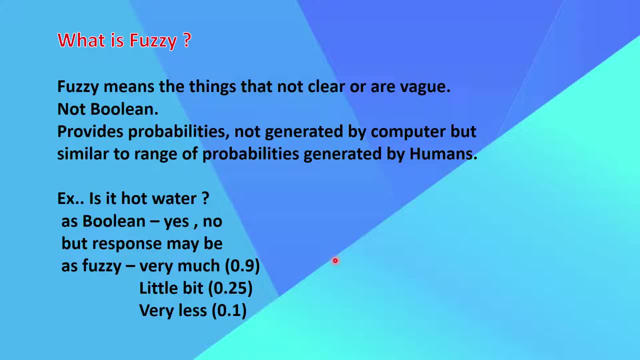 be very much, little bit or very less. So it provides the probability not generated by the computer but similar to range of probability generated by humans. So we can assign some probability here, like here: very much has a probability, highest probability, like 0.9. 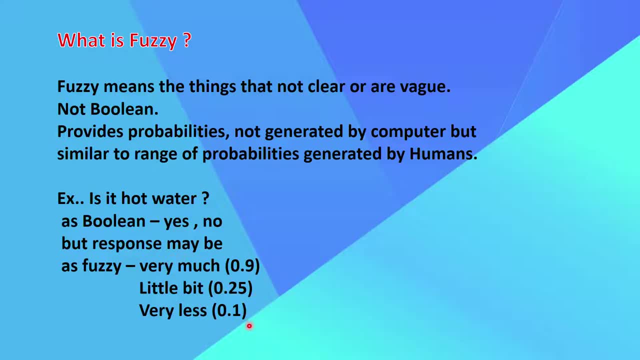 and the little bit has a probability 0.25 and very less has a very low probability like 0.1.. So we are not going to do anything much. We are just trying to assign some probability in the range of 0 to 1.. 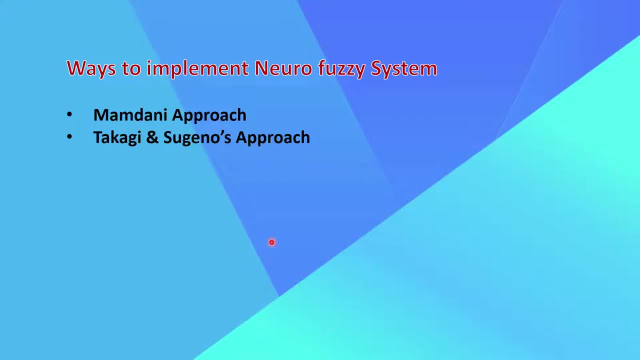 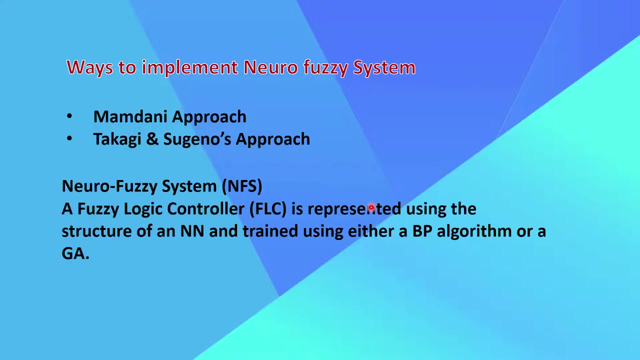 So there are two ways to implement the neuro fuzzy system. One is the Mamdani approach and another one is Takagi and Sugeno's approach. But we are only considering Mamdani approach here. So before going ahead, let's see actually what exactly neuro fuzzy system is, So neuro? 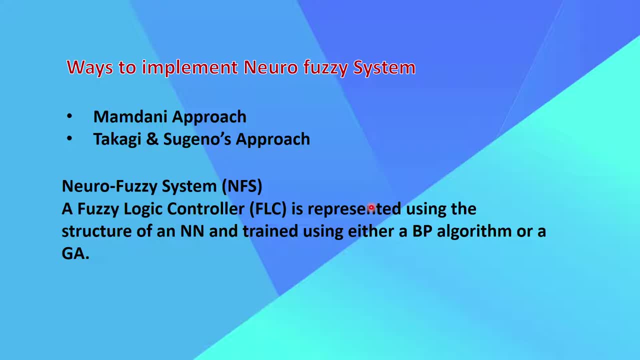 fuzzy system is something which is the fuzzy system which is trying to be represented in the structure of neural network, And we are going to train it using either wave propagation algorithm or genetic genetics algorithms. So I hope till now you got the at least basic idea of the 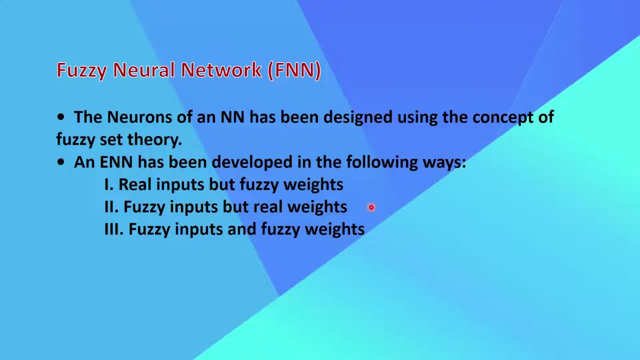 about the neurofuzzy system. now, if we have a neurofuzzy system, then why not? we cannot have a fuzzy neural network, as in which we can. the neurons of a neural network can be implemented or designed using the concept of fuzzy system. maybe where can the possibilities like real? we can use a real input weights in the. 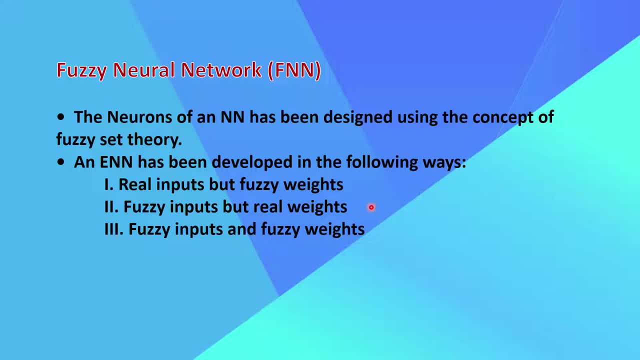 neural network and the fuzzy weights and fuzzy input, or real weight or or we can use a fuzzy input and fuzzy weight. there is no sense to use a real weight and real inputs because of it will become a simple neural network. the fuzziness will be not there. so we can also make a fuzzy neural network by 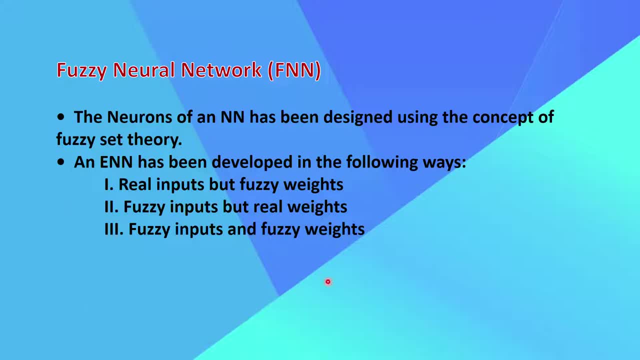 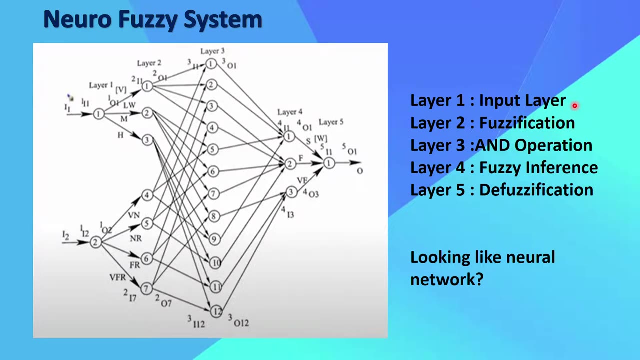 using this particular three approaches, but- but due to some bad luck, probably what we can see, but this approach is not got that much property, so that's why we are following the new fuzzy system. so let's take a deep learning. in the mamdani approach there is, there are three extra layers, or 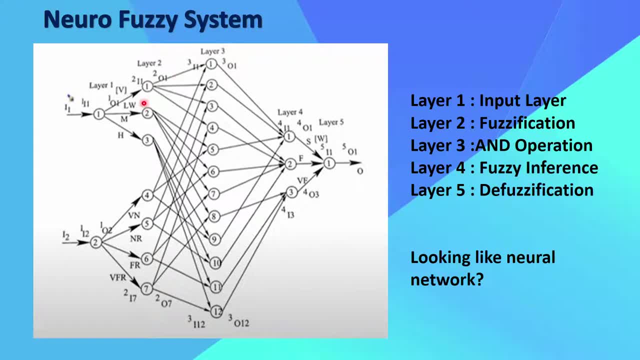 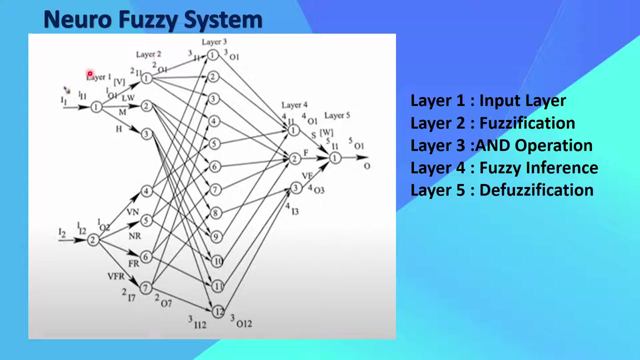 the hidden layers with, along with the two input and output, put layer. so let's look, look at here. this diagram is more looking like a neural network, but it is not so there we are having two inputs and at the layer one and layer two we have a facification process that we are going to apply over 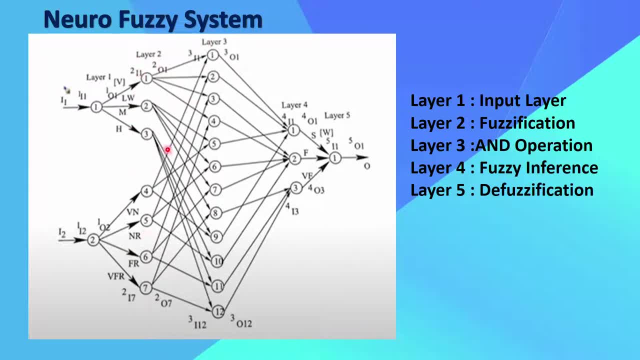 here we are going to apply some membership function or any, some two, they're going to convert the for the fortification process. and layer three- this is a end operation layer. we are we are going to perform end operation on a fuzzy, fuzzified values. and at layer 4 we have inference engine, a fuzzy inference. 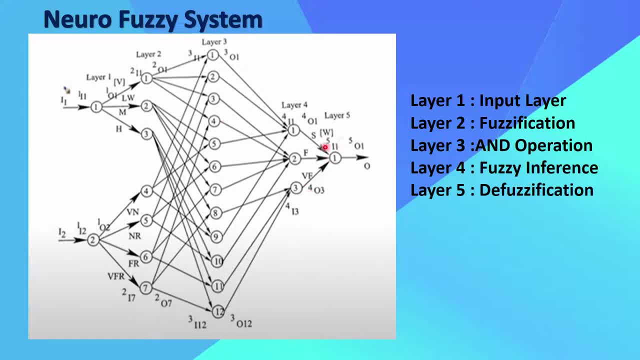 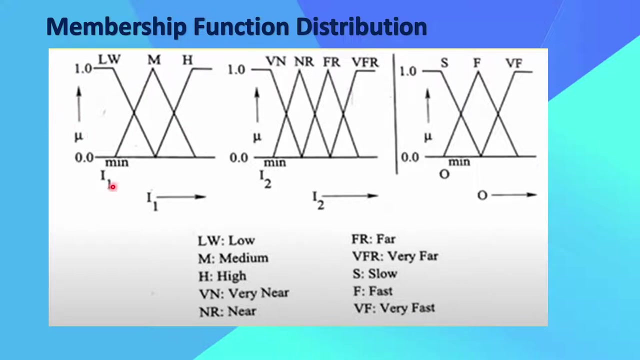 engine And layer 5, we are going to defacify the output that we are going to get So that we can convert the input into crisp values. So let's see, for example, as we are performing a membership function in the fuzzification layer. So there are two inputs, as I said. 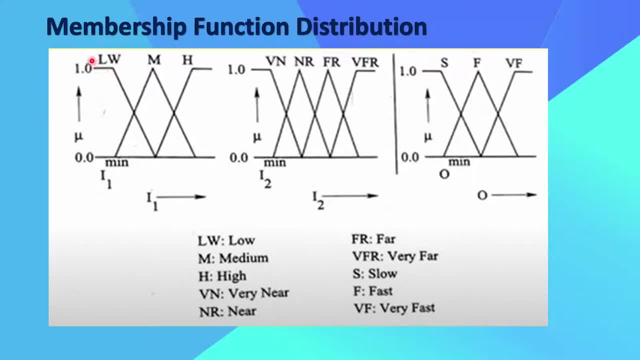 After the fuzzification, the values that is passed as input, going to convert as a low or medium high and very near, near, far, very far. As also at the output side We have a values like a slow, fast, very fast. 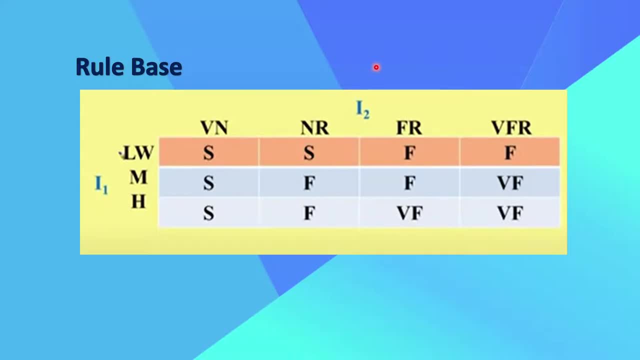 So, before going ahead, I just want to discuss some of the components of fuzzy system and how exactly the fuzzy system works. Actually, in the process of fuzzy system, there is some steps. We are passing our inputs in the form of crisp values. 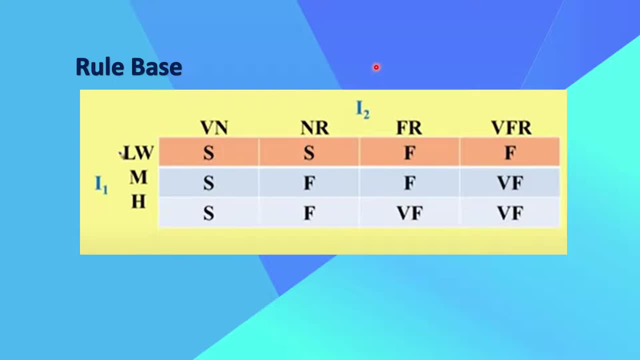 And this particular values are passed For the fuzzification process so that the some membership functions are applied over there, And there is something known as rule base which is connected with the inference engine. So the rule base contains some rules, or we can say if-then rules. 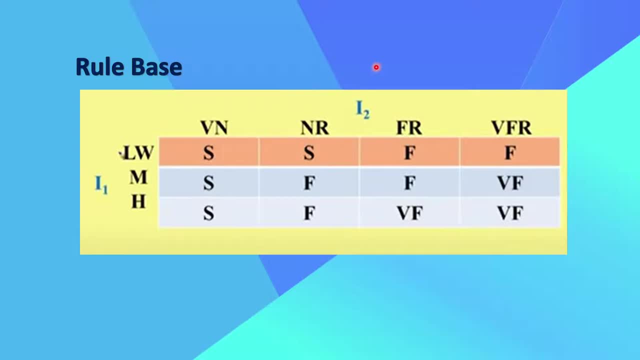 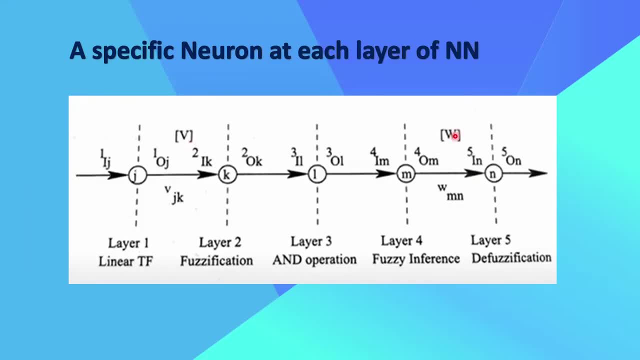 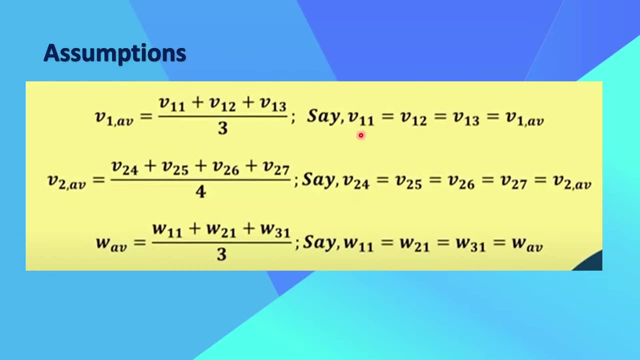 as I have shown here, We are going to take the average of all the weights. We are not considering the separate weight for each branch or neuron. We are taking the average weight of all the nodes At the output side. we are also considering the average weight, just for. 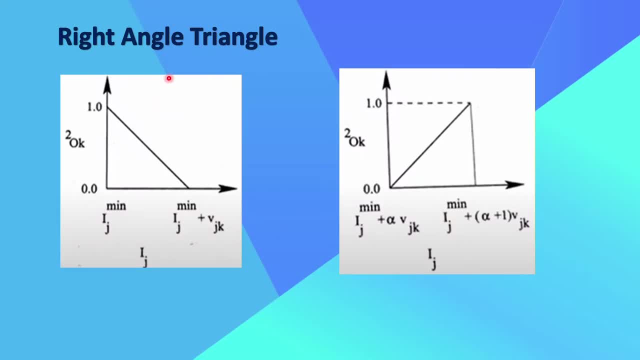 a similarity purpose. So at the falsification process we are considering that the right angle method or triangular method is applied. I am assuming that the angular and triangular method even know about this. So what we are going to do here in the triangular method?